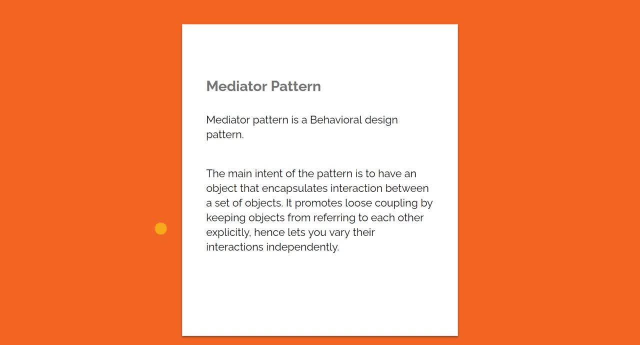 coupling by keeping object from referring to each other explicitly. Hence lets you vary their interactions independently And just like. like any other behavioral pattern, the main intent of this pattern is also same: It is about loose coupling between multiple objects. Now, as you can understand by its name, Mediator Design. mediator means someone who mediates. 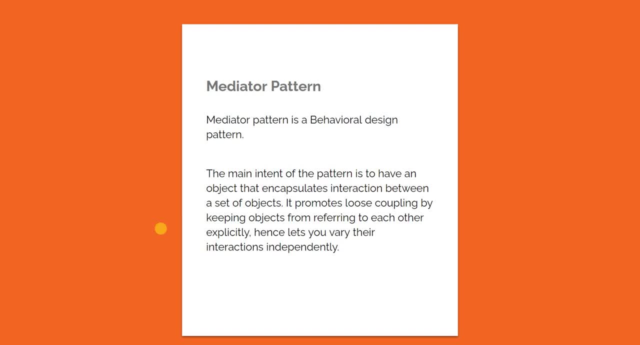 So a classic example for mediator design pattern is chat software, where everyone connects to chat software And when the chat messages to each other. the chat software manages the code of the Sophia disk. But it can be done with little effort as well, So I will show you how I. 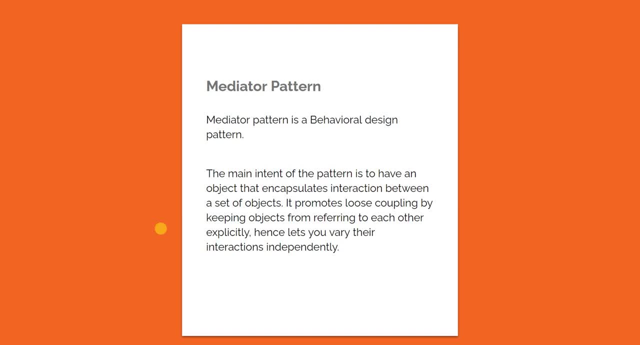 work here might be faster if I have two, so that I know what you are thinking while talking- some communication between the two objects instead of the objects talking to each other peer-to-peer. But in today's video I'm going to take a different example. Another example that comes in mind is 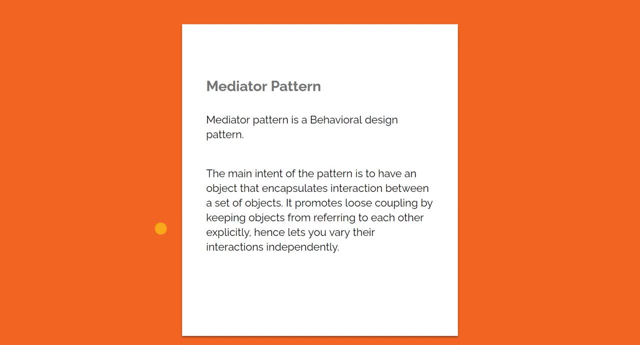 before we had Uber or Lyft, usually we used to book cabs using a cab company, So there are multiple cab companies and the way it works is: when we book a cab, we call a call center. Someone in the call center responds to the call and then they figure out if a cab is nearby my 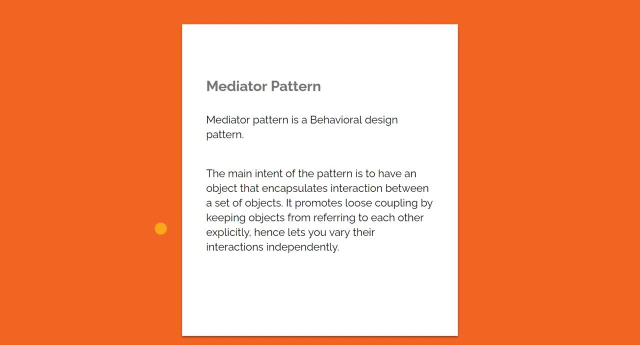 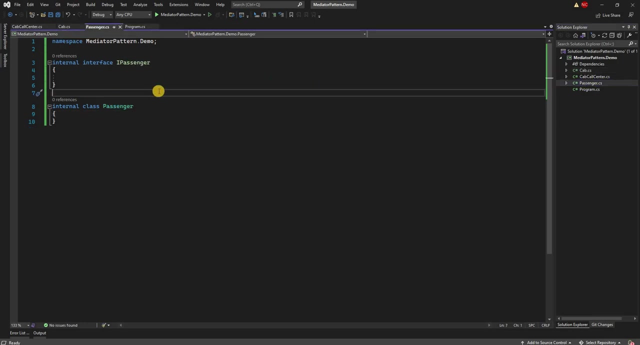 area and then they send the cab to my house. That's how usually a call center based cab system works. Today we'll try to program this particular system. So for that, what we are going to have is: we are going to have a cab class, which will be representing a cab. We are going to have a 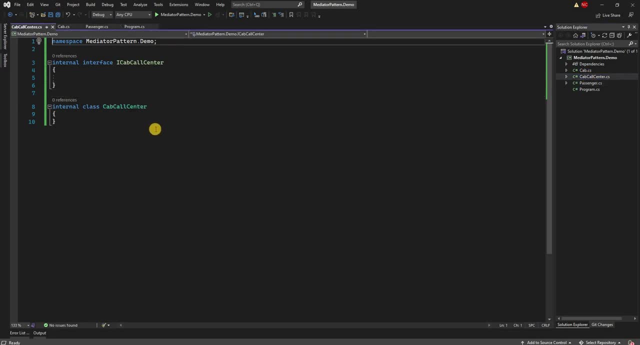 passenger class, which will be representing a passenger, and then we are going to have a call center, which is going to represent a call center. Now for the call center. we'll start with call center. So what is the responsibility of a call center? First responsibility is every cab. 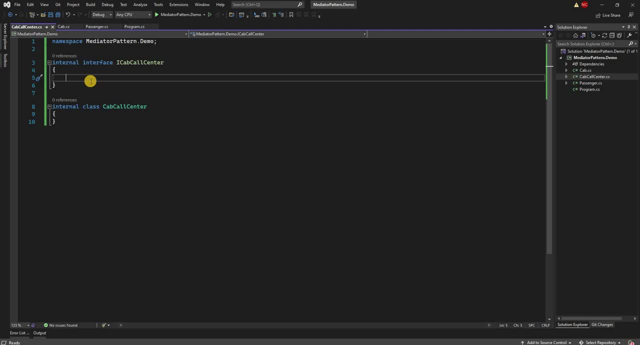 is going to register itself to the call center, So we can have register and the registration is going to happen based on a cab And the second responsibility is a passenger calling To book a cab. So we can have another method called book cab and we can have I passenger as the parameter. So now we can implement the 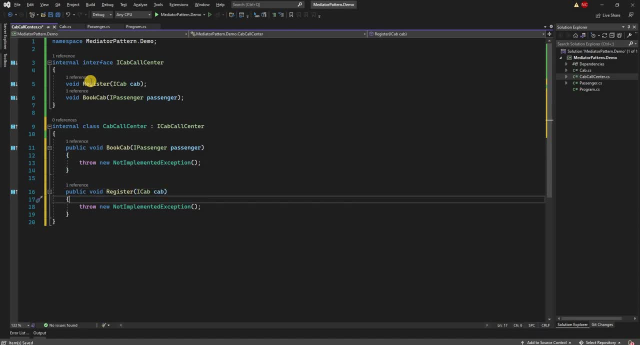 cab call center. So let's first implement the register, and the registration is going to be straightforward. So for registration we need a dictionary of cabs. So what we can do is we can declare a private, read-only dictionary of the name and the cab And we can call it as cabs, and this is going to be. 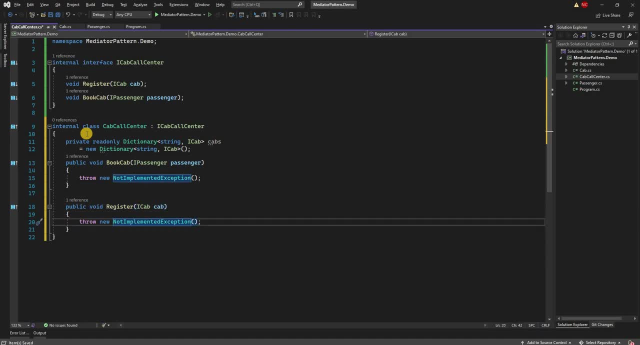 equal to new dictionary of cabs. And on registration, what we are going to do is we can check if cabscontainsvalue of the cab. So if it does not contain, then we can say cabsadd and here for the name we can say cabname and the cab itself. So we need to create a name: property in the cab. 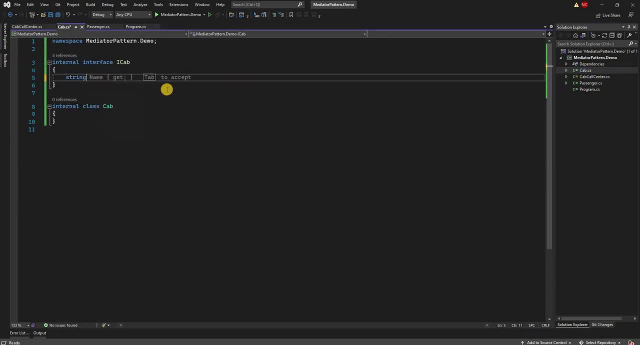 So let's go back and here let's create a string name. That's one property. The other thing also we would need for a cab is its current location, And usually the current location is going to be in the form of a latitude and longitude. 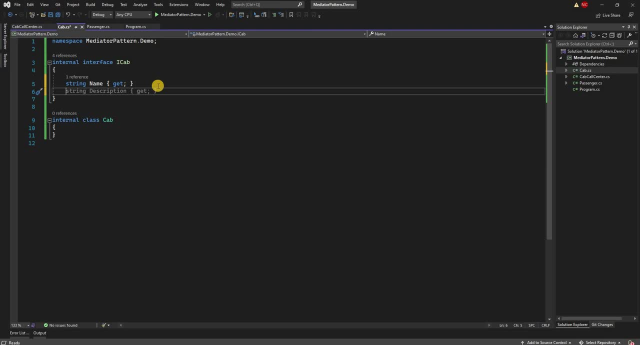 And based on latitude and longitude, we can find out the latitude and longitude of the collar and we can do some geometric calculation to find out how far the cab is from the location of the collar. But for simplicity, what I'm going to do here, I'm just going to use an integer value. 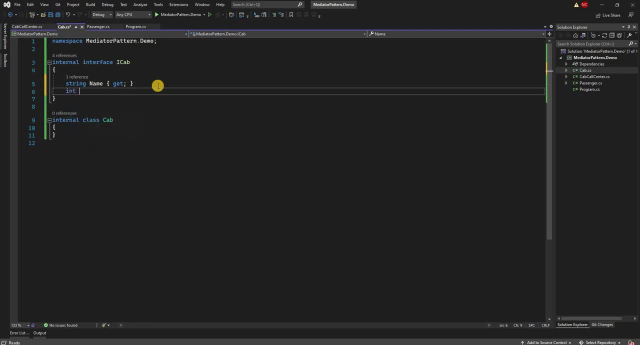 So that we can do simple math. So here we can have something called current location. Current location can be again a get. And the third property that we need for a cab is if the cab is free or not. So let's say bull is free. 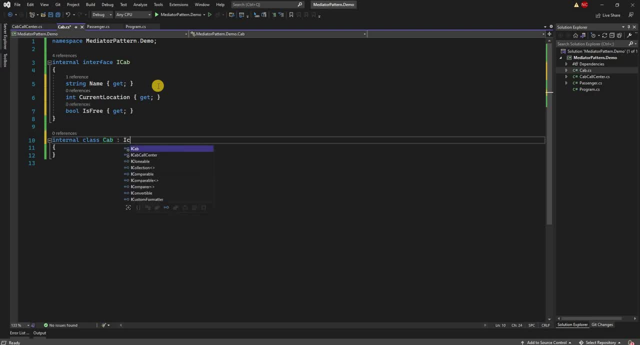 So this is the three properties, and then we can implement icab And here we can have private read only string name. Private read only int location. Private read only bull free. And then for name we can just send the name For the current location, we can just 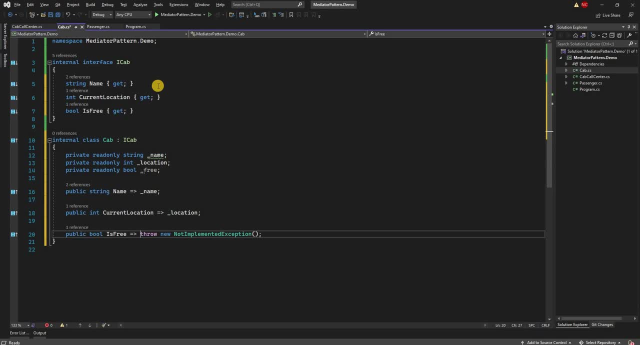 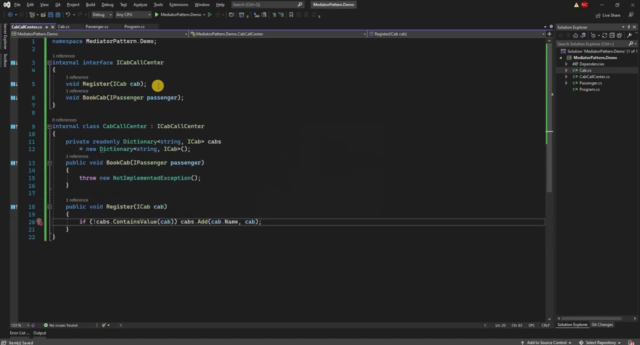 send the location And for the free, we can send the free. So this is the three properties we are going to use for the cab. So the cab is now added And then what we have to do is when a passenger calls to book a particular 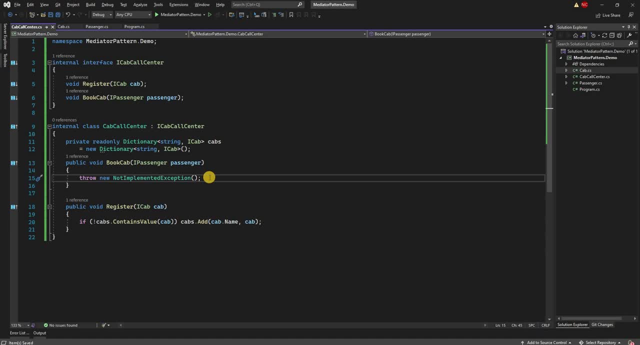 cab. what we want to do is we want to go through all the cabs And the cabs which are currently free, And then what we are going to do is we will be finding if the cab is within a certain radius Of the passenger's location And if it is, then we are going to assign the cab to the passenger. 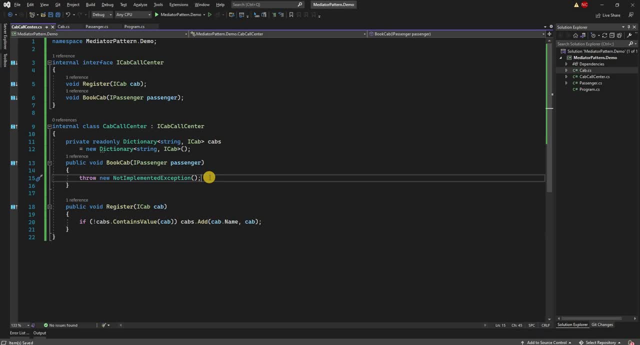 And then we will let the passenger know that we have assigned. So if we have to do that, what we need is we need a private function So we can have a private bull is within, let's say, five mile radius. This radius can be a parameter. We really don't have to say five mile, But for 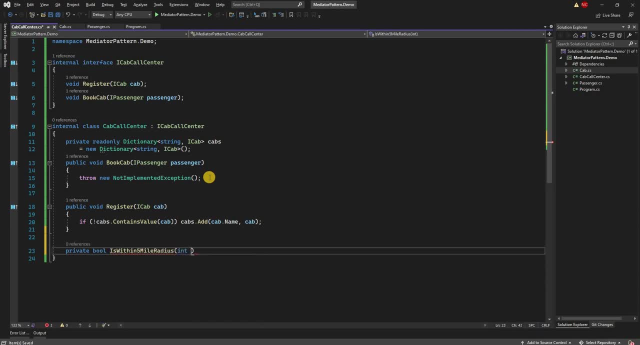 the example here. I'm just figuring out five mile And, as I mentioned that, we are using int as the current location instead of actual let long Just for the simplicity of showing the calculation. So we can have the cab location as the first parameter And then 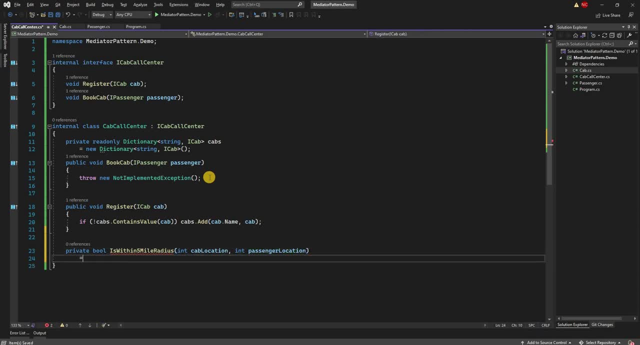 passenger location at the second parameter. And in this method all we can do is we can do math, dot absolute And we can say: cab location minus passenger location is less than five. So if it is less than five mile, then the cab can be assigned. 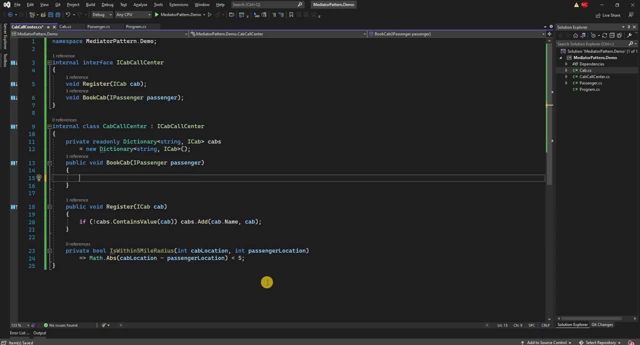 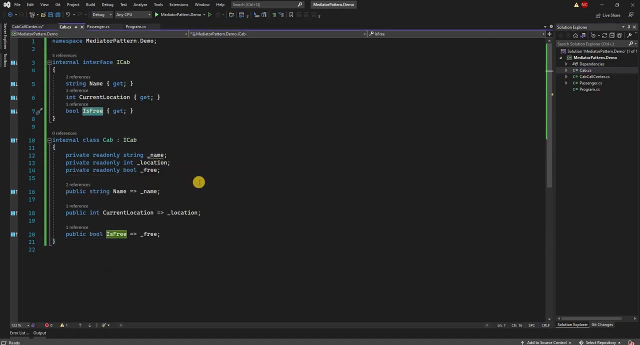 So here what we can do is now we can come here and we can create a for each loop And we can say for each cab in cabs dot where the cab is free. So for the cab we have, the is free, I have to do cab dot values. 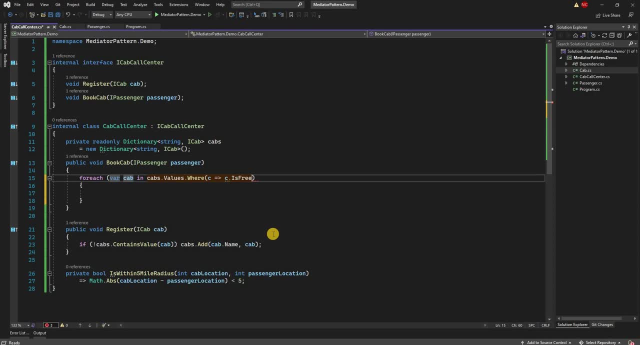 dot, where cab dot is free, And then for each of the cab we can say if is within five mile radius, And we can send the cab location. So we can say cab dot location which is current location, which is an integer, So we can say if. 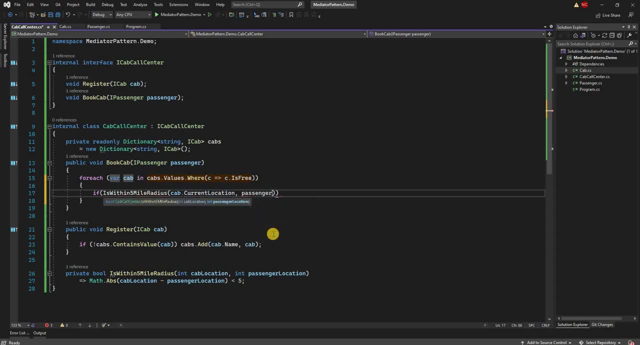 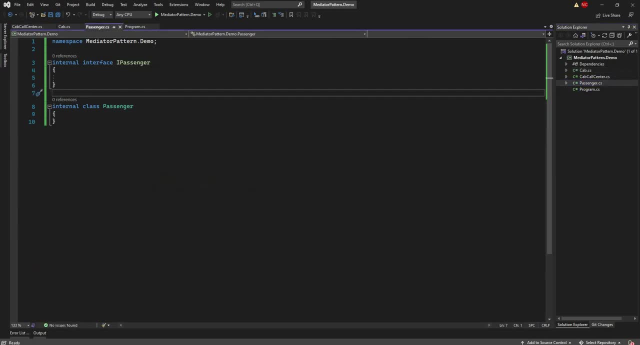 then we will send passenger dot location. So let's go and create some of these parameters for passenger also. So for passenger we are going to have name, because the passenger will have a name, then the passenger will have address and then, finally, passenger will have location and we can implement the. 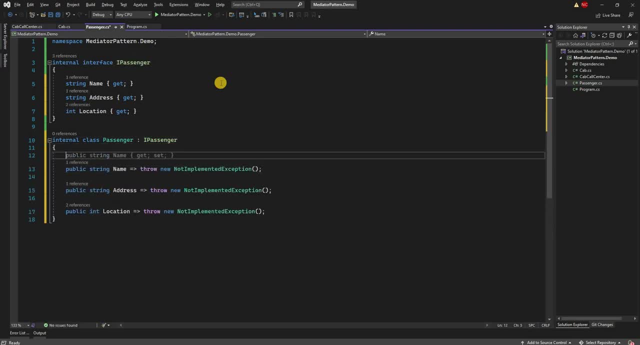 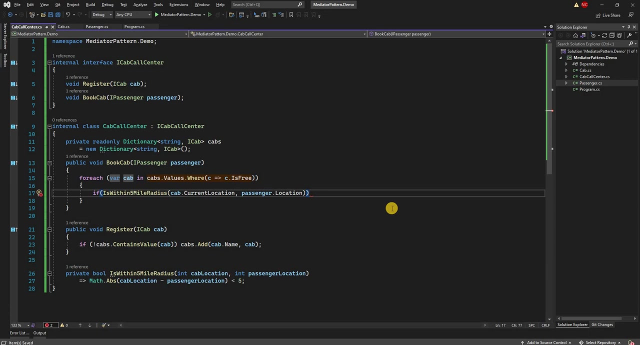 ipassenger here and similarly we can have private string name, private string address, private string location, and here we can send underscore name. we can send the underscore address and here we can send the underscore location. so this will figure out if the address of the cab is within five mile of the passenger. 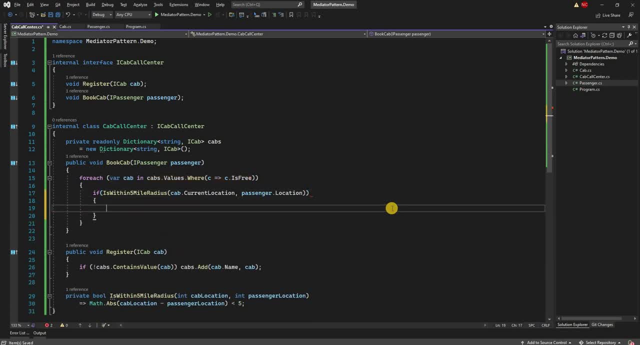 and if it is, then what it is going to do is where it's going to say: okay, because it is within the location. it is going to assign the passenger to the cab. so it's going to say: cab dot assign. we are going to create a assign method and it's going to take the passenger dot name and 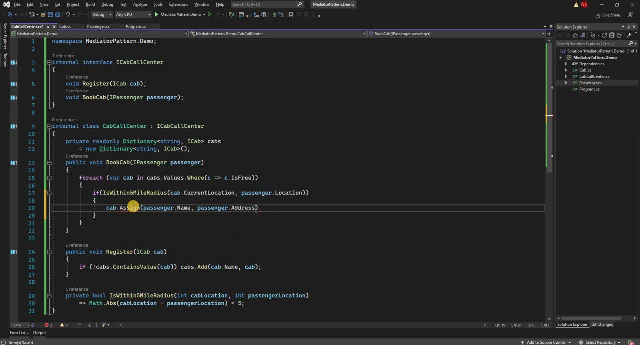 passenger dot address, these two parameters and then after that it's going to inform the passenger. so it will call a method called acknowledge and here it's going to send the cab dot name just to say which cab is is assigned. so we're going to generate this method in icab. generate method in. 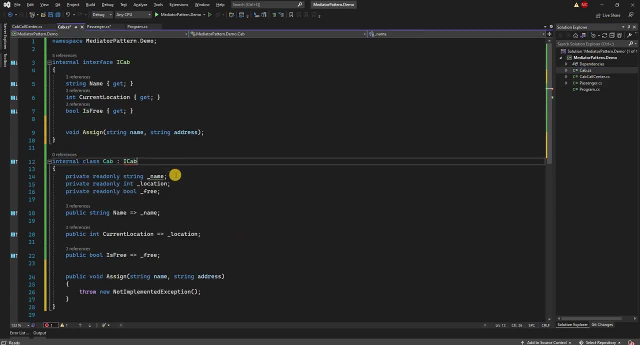 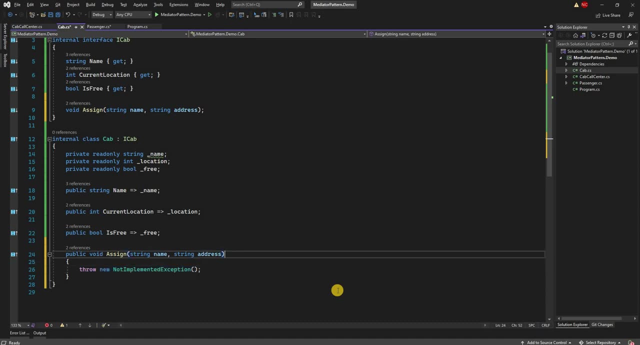 ipassenger and let's go here and let's implement this method. and here the implementation is going to be simple. we're just going to have a console dot write line so we can actually make things simplified and we can say console dot write line and we can say cab. 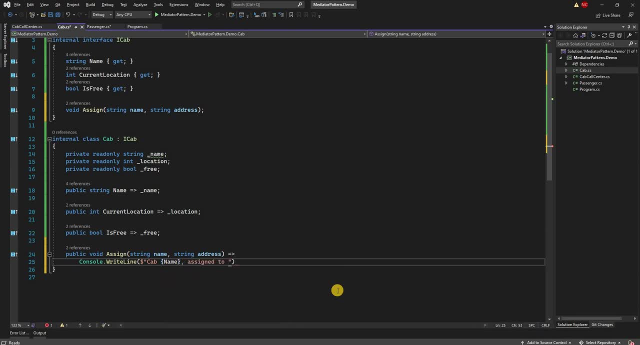 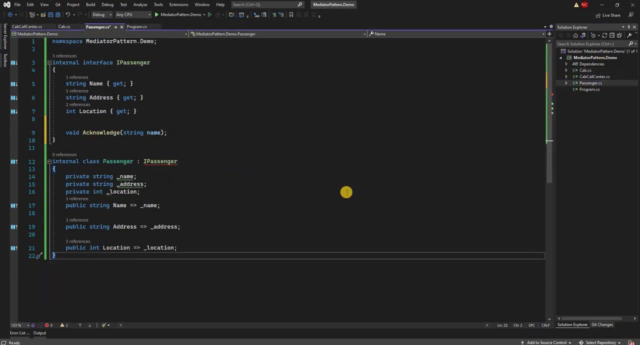 name sign to passenger and we can say the name of the passenger and address of the passenger. as simple as that, nothing fancy here. and then, similarly, we can go into passenger, we can apply the acknowledge and in acknowledge also you can have a simple implementation. so you can have a console dot write line. 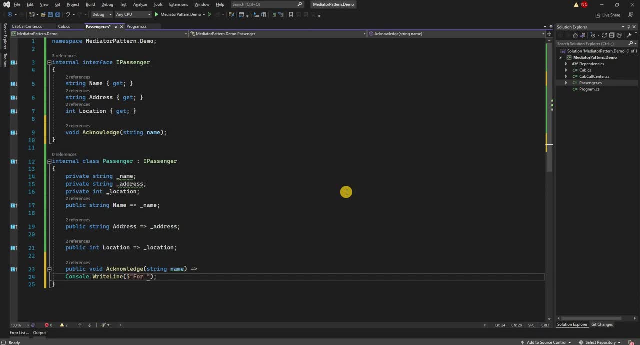 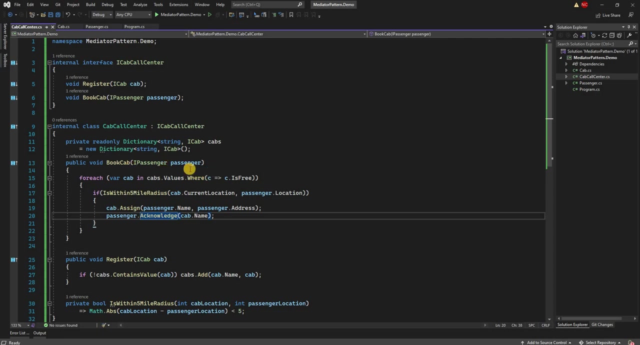 and we can say here: for passenger name, cab name, name of the cap, just simple print statement. so now what is happening here is when we get to the call center, when a call comes into book, we get the passenger info and then we we iterate through all the caps and find out if the cab's location 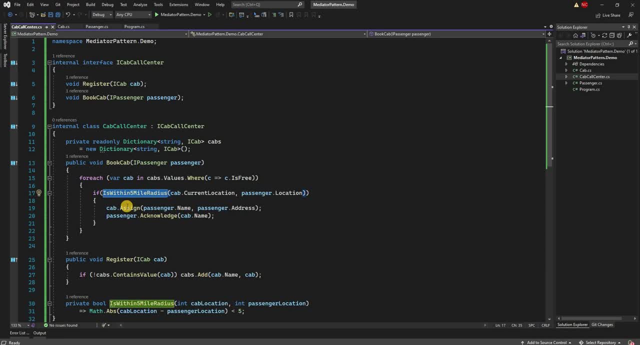 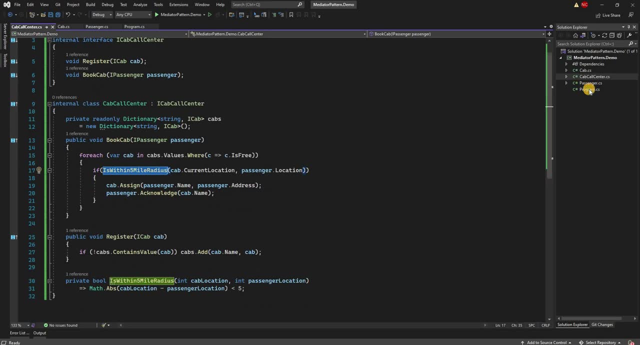 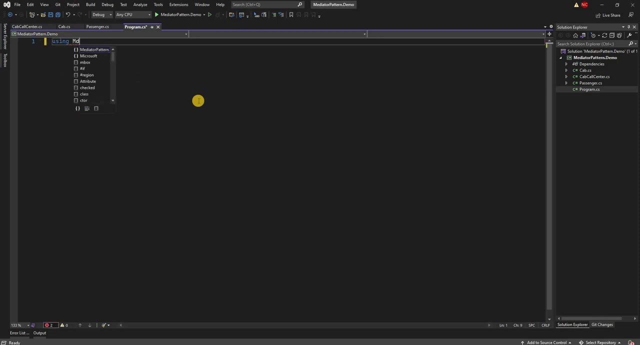 is within the five mile radius of the passenger, and if it is, we assign the cab and then we acknowledge the passenger with the cab name. so this is the whole implementation, and then now what we can do here is first, let's do using mediator pattern dot demo. 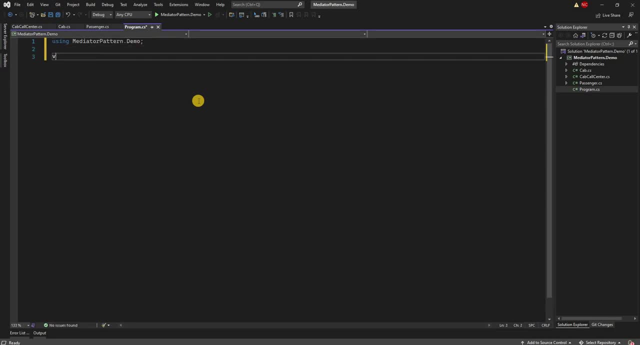 set the namespace because we need this. so first we can do is var call center is equal to new call center, cap call center. and then what we can do is we can create the passengers. so let's say we have a couple of passenger so we can say passenger one equal to. we have to provide constructor. 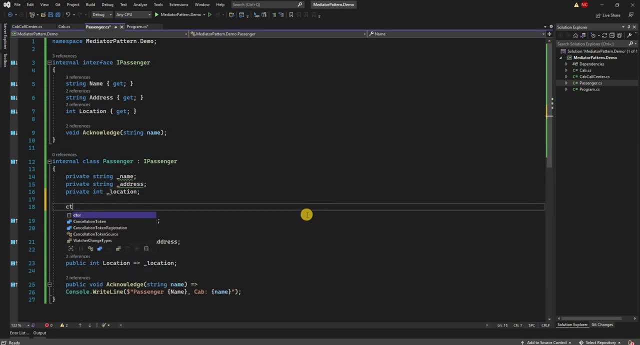 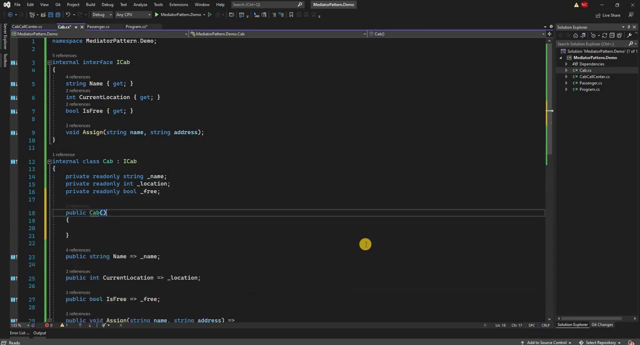 to set the name, address and location. so it will be VAR. so sure, okay. and similarly, we have to do the same thing for cab. so let's create a constructor and we can have string name- location is free and we can assign the values in the constructor. so now 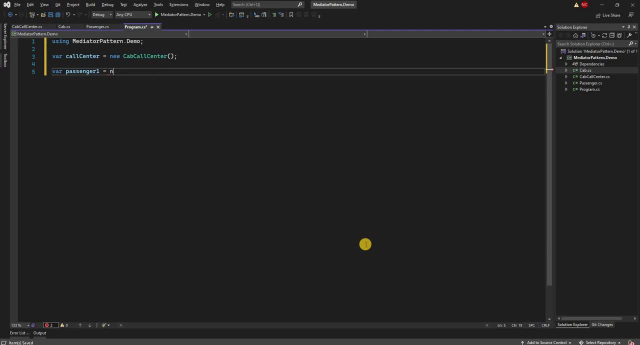 here we can say passenger is equal to new passenger. and for the name we can say this passenger one. for the address we can say one to the street. and for location we can say 10, let's say 10 is the location, as I said, just for. 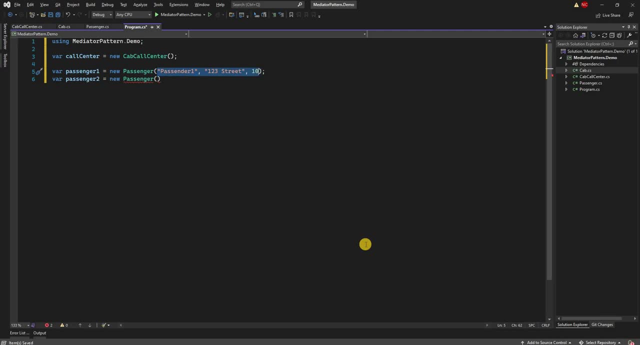 simplicity, I gave integer, but for real-life scenario this will be a latitude and longitude, passenger two, and passenger two is a location of 25, and then let's create cabs, so cab1 equal to new cab and the name is cab1. and then the location, let's say, is equal to 11 and free is equal to. 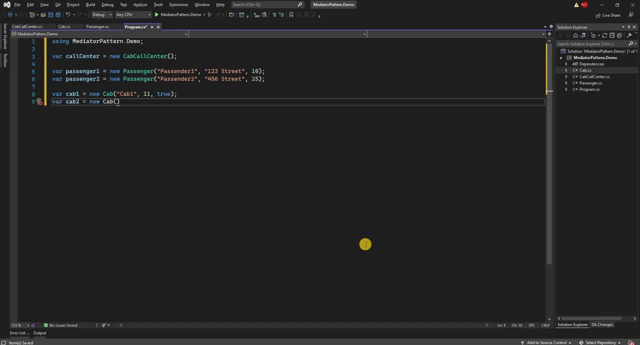 true, and then we can have cab2. cab2, the location, let's say it's 22, and this one, let's say right now, it's false, it is not free. now we can register both the cabs to the call center and cab2, and then we can book cab for passenger one. 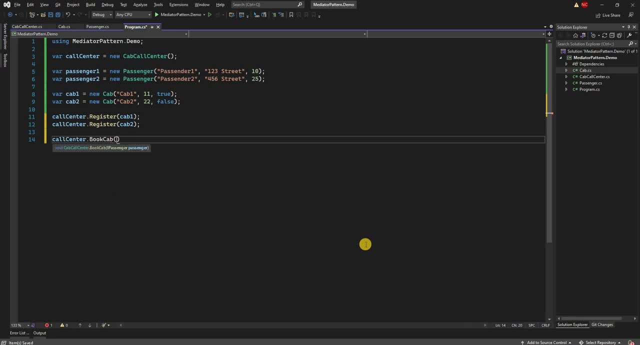 and passenger two. and finally, we'll just do a console dot read line just to wait for the function two execute and stay there. So now, if we run this application, what is going to happen is the mediator, which is the call center, will get a call from passenger1 and passenger2.. 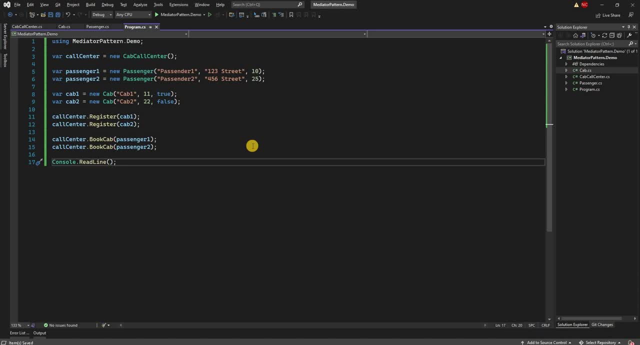 For passenger1, it will find out that cab1 is available and it is within the range, so it will assign cab1 to the passenger and acknowledge, Whereas for the passenger2, though, the cab2 is within the range, but cab2 is not free, so it is not going to assign anything. So if we run this, 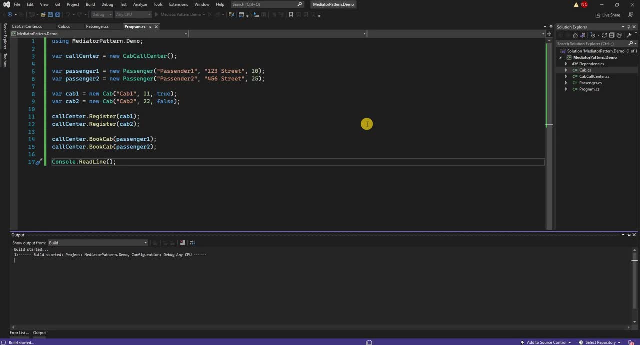 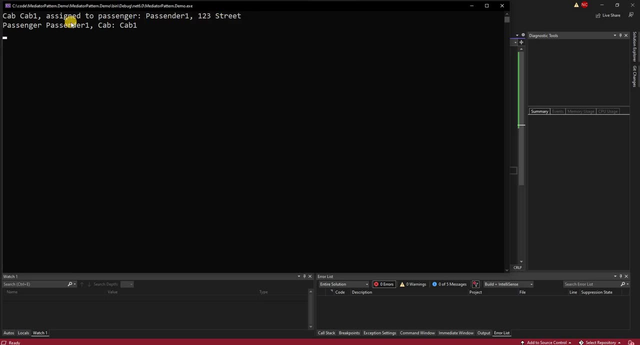 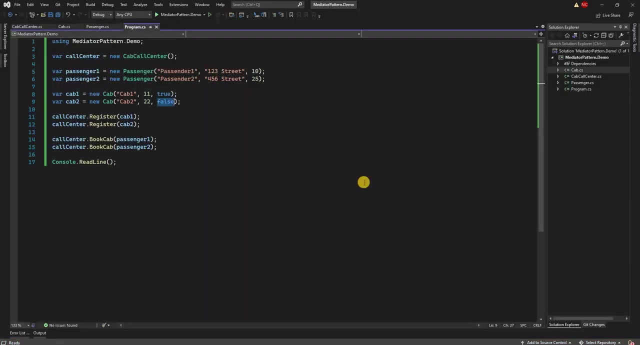 we should see only one printout for passenger1 and cab1.. As you can see, cab1 assigned to passenger passenger1 and address is 123 and passenger1 got an acknowledgement that cab1 is assigned to the passenger And now, if we make this as true, so both of them are free now. passenger2.